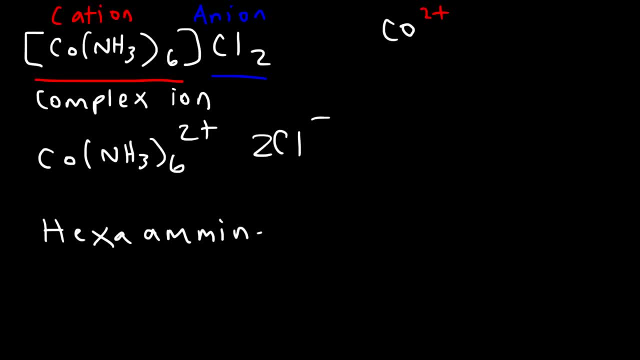 When you name it, you need to use two M's as opposed to one. So this is going to be hexa amine, And then we need to name the transition metal, cobalt, And then the oxidation state, which is two. 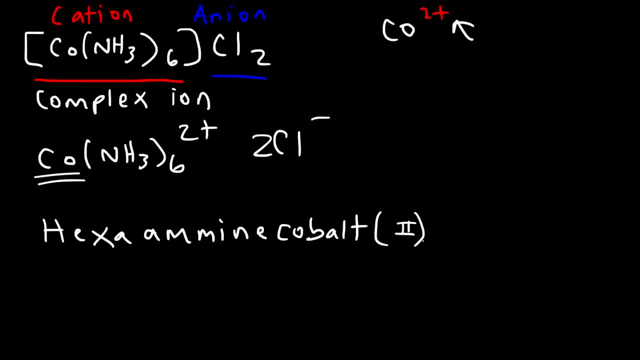 So the name of the complex ion is hexa amine cobalt two, And then we can name the anion. We're going to use an IDE ending, So that's simply going to be chloride, And so that's how you can name this particular coordination compound. 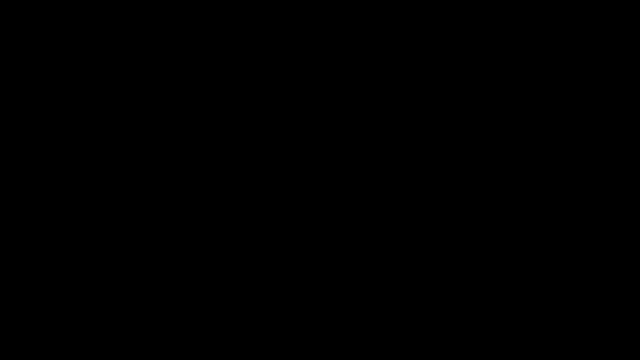 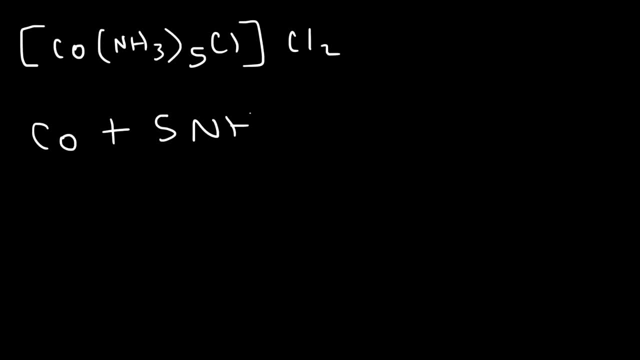 So we have CO, five NH3 molecules and three chlorine particles. Now ammonia has an oxidation state of zero, Chlorine is negative one, And so it's going to be X minus three is equal to zero, So X is three, So the oxidation state of cobalt is plus three. 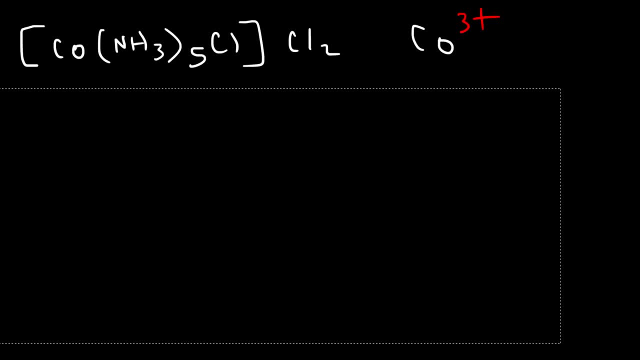 And so we're going to calculate the oxidation state of cobalt. Now let's go ahead and name it. So let's start with the complex ion first. So we have five NH3 molecules, So five stands for a penta, So it's going to be penta amine with two Ms. 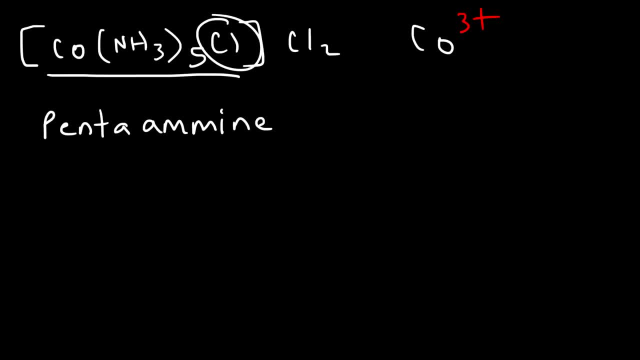 And then we have a chlorine. that's part of the complex ion, So we're going to call that chloro, And A comes before C, So we need to put it in alphabetical order. And then after that it's going to be cobalt, with an oxidation state of three. 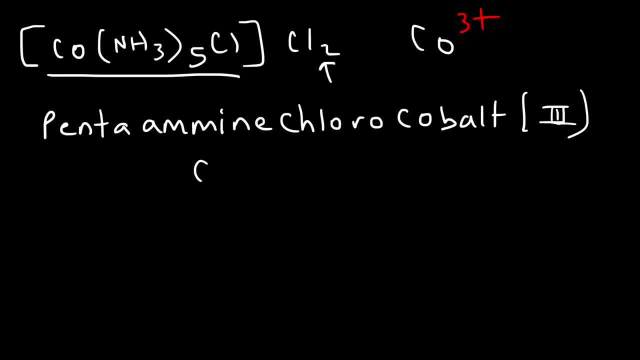 And then we can leave a space, And then for the anion we're just going to say chloride, So it's penta amine chloro, cobalt, three chloride. Now let's move on to our third example. Go ahead and try that one. 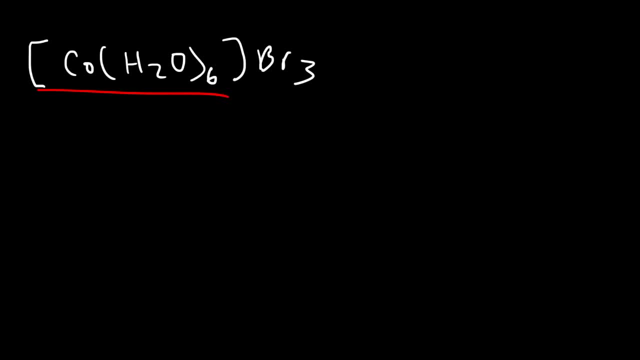 So, once again, the complex ion is three, And the complex ion is the cation. Now let's determine the oxidation state. first. The oxidation state of water is zero And for bromide it's negative one. But there's three of them. 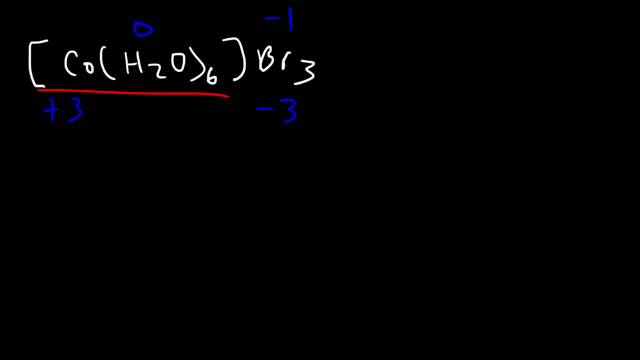 So this is going to be negative three, which means cobalt has to have an oxidation state of plus three. If you don't like that method of doing things, you can write the equation to get the answer. Now let's start by naming the complex ion or the cation. 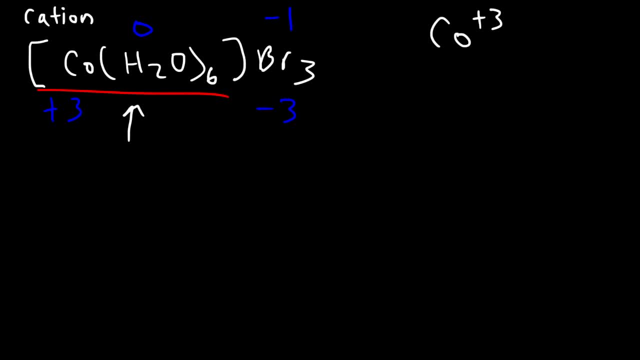 So what is the prefix for water? What's the name for it? When dealing with water, you need to use the word aqua, And there's six of them, So it's going to be hexa aqua. Aqua means water. 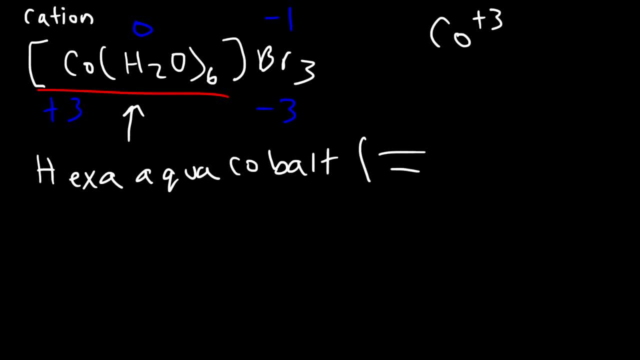 Cobalt with an oxidation state of three. And then the anion is bromide. So instead of saying bromide, just replace the ine with ide. So it's hexa, Aqua, cobalt three. Well, I put bromine. 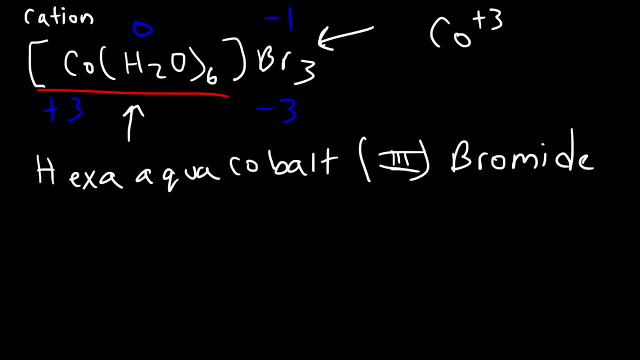 This was supposed to be bromide. Hexa, aqua, cobalt. three bromide, Let's try this one. K3, Fe, Cn, six. So this time, notice that the anion is the complex ion. 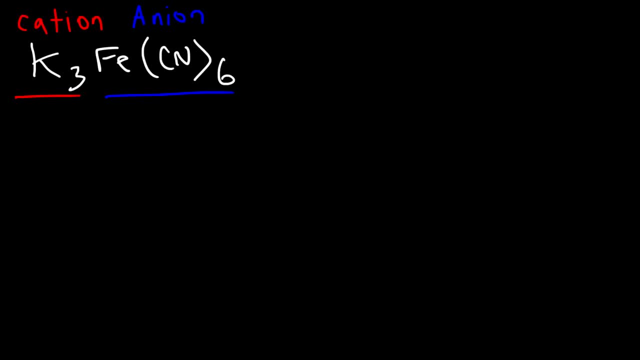 So the name is going to be a little bit different in this example. But first let's calculate the oxidation state of Fe. So we have three potassium atoms or ions, And then we have Fe and six cyanide ions. Now the charge on potassium is going to be plus one. 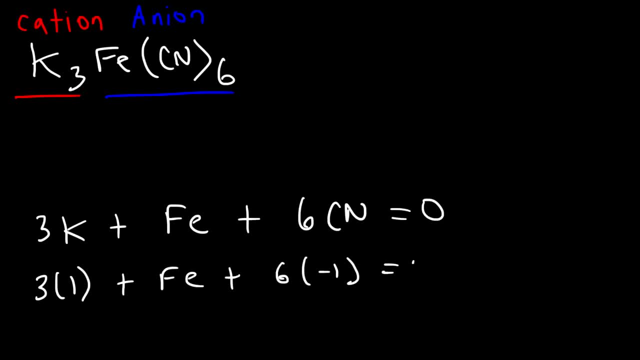 And for cyanide it's negative one. So this is three And then this is negative six. So we can combine like terms: Three minus six is negative three And then if we add three to both sides we can see that the oxidation state of Fe is positive three or three plus. 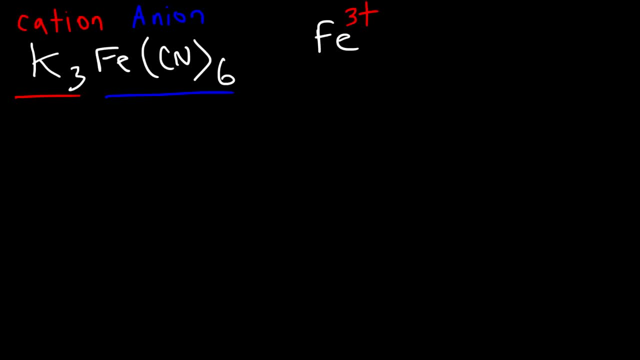 So, now that we have the oxidation state, how can we name it? The first thing you should do is name the cation And you just got to name the element. So the element K is potassium. So next name, the complex ion. 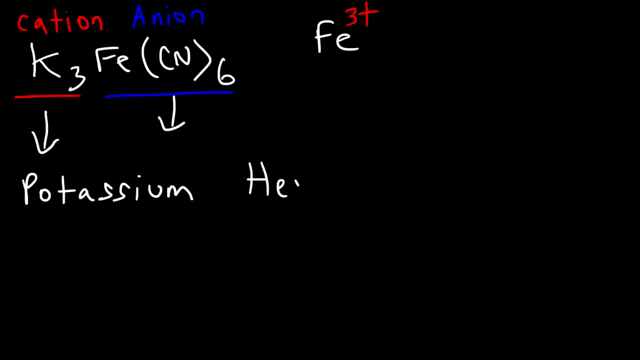 So we have six ligands. So it's going to be hexa, And for cyanide as a ligand you would call it cyano. And then to name Fe, you won't say iron, But you have to use the Latin name. 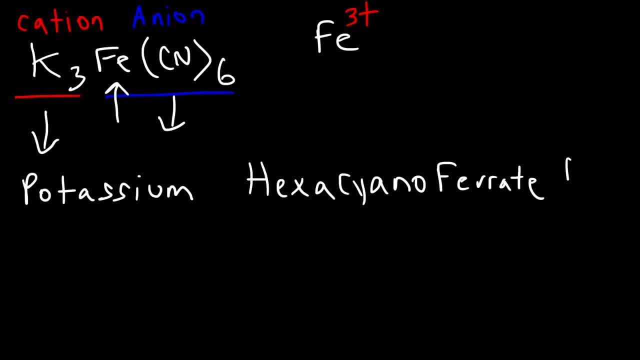 So you would say ferrate, And then the oxidation state, which is three. So it's potassium hexa, This is cyano ferrate three. Now let's move on to the next example, K3COF6.. So, once again, the second one is the complex ion. 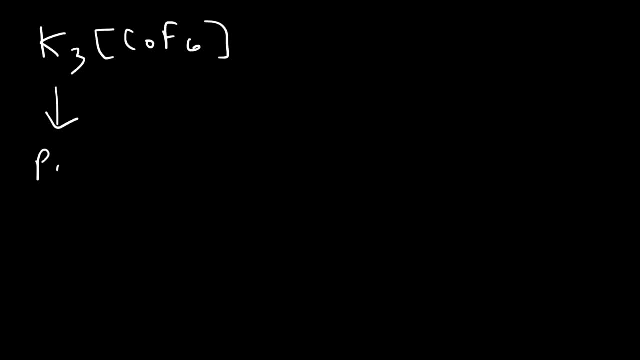 So first let's name K- K is potassium- And let's identify the oxidation state. Potassium has a plus one charge, Fluorine has a minus one charge. One times three is three Negative. one times six is negative six. 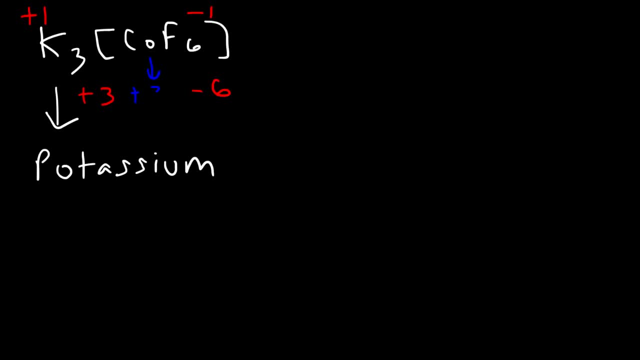 Now cobalt has to have a plus three charge So that these three numbers add up to zero. So once again we have the cobalt three plus ion. Now let's go ahead and name the complex ion. So we have six ligands. 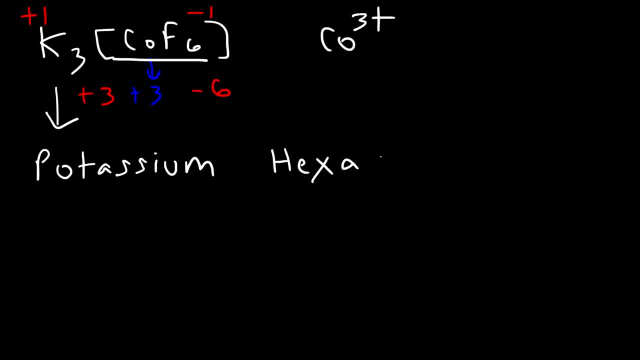 Therefore this is going to be hexa, And the ligand is fluorine, So we're going to call it fluoro, And then the Latin name of cobalt, which is cobaltate, Then the oxidation state three, So it's called potassium hexafluoro cobaltate three. 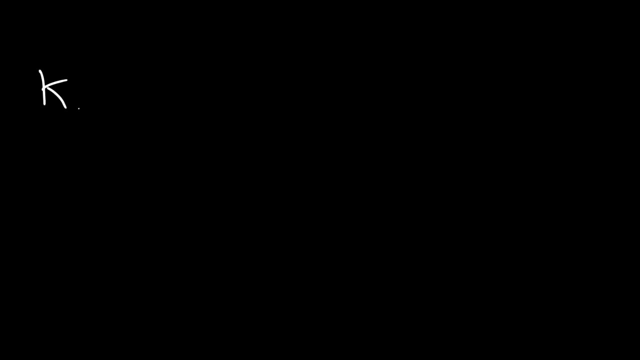 Now let's try one more example, And instead of using K, let's use Na, So Na4PTCl6.. Feel free to pause the video and try this. Sodium has a plus one charge. Chlorine has a minus one charge. 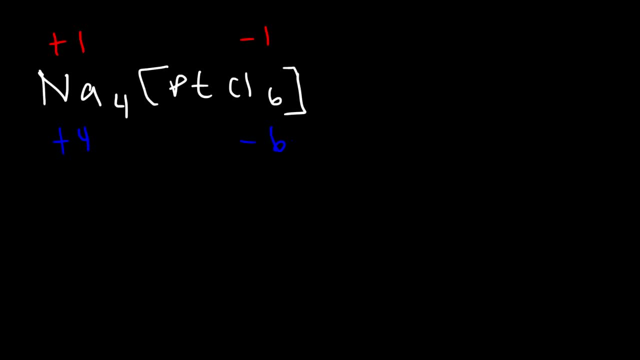 So this is going to be plus four, minus six, And for these numbers to add up to zero, platinum has to be plus two. So now that we know the oxidation state of platinum, let's name it So Na is called sodium, And now let's name the complex ion or the complex anion.